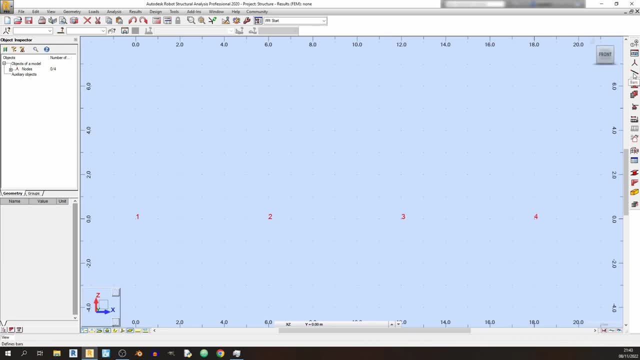 here. So we're going to need to draw in the bar elements that connects all of our nodes here. To do so, go to the bars button over here, right underneath the nodes over here, and change the bar type from simple bar to rc beam, and by default you should have quite a few options. 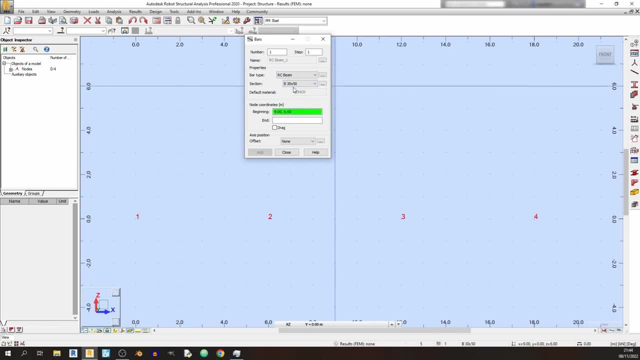 here for your sections. So for this tutorial, I'll be showing you how to create a new section type. All you need to do is just click on this box here with the three dots over here, and a pop-up window will emerge titled new section. So right now we are using a rc beam section type and you can 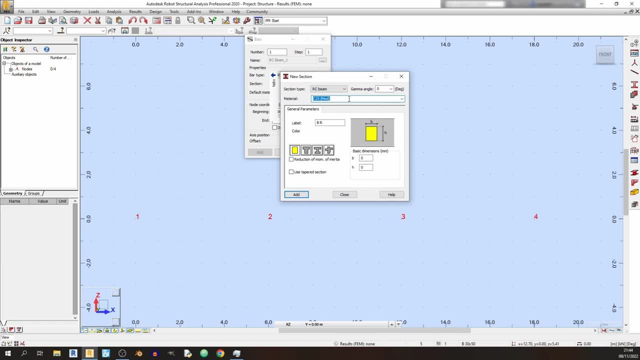 select the material strength for your reinforced concrete beam. So I'll just leave it as c25 for now and the breadth for my beam in this tutorial would be 300 millimeters here and the height would be 600, and I'll be using a rectangular beam over here and you might have noticed that robot structural. 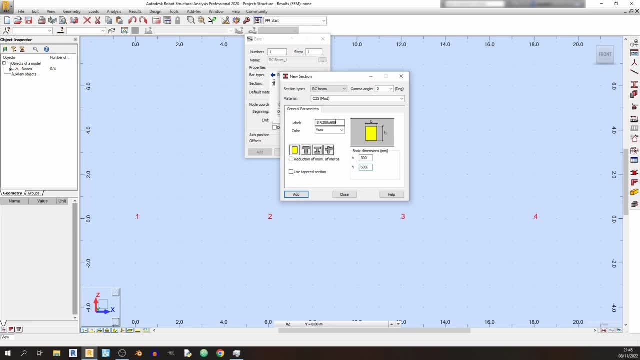 classes made a custom label already, So this is based on the breadth and the height of the beam. So click on add and close and I'll select this 300 by 600 beam over here and I'll draw from node 1 to node 2, node 2 to node 3 and node 3 to node 4 and click on close and to view the member itself all. 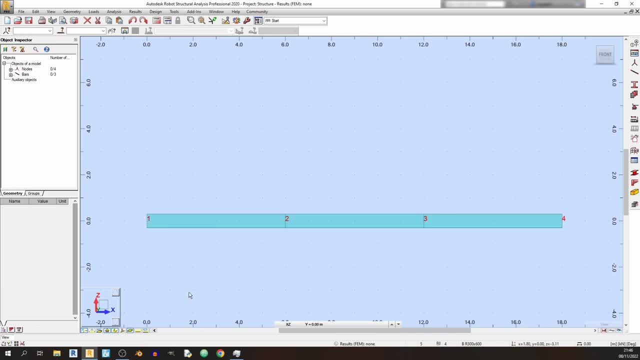 you need to do is select this section shapes over here and you can see it in 3D, like so. If you want to go back to the original view, you can just click on front, like so, and you can turn it off. as it's not, 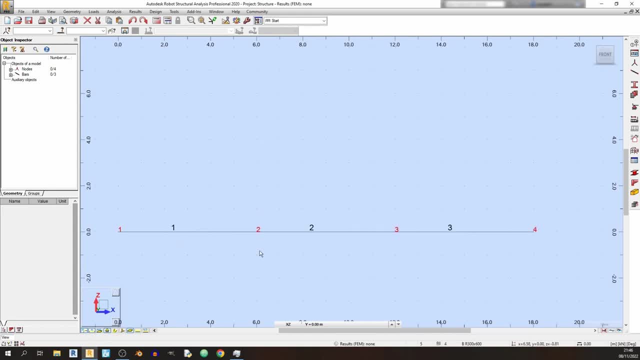 needed for now. If you want to go back to the original view, you can just click on front, like so, and you can turn it off, as it's not needed for now. But you can turn on bar numbers over here so you can see that we have three bars over here, So a. 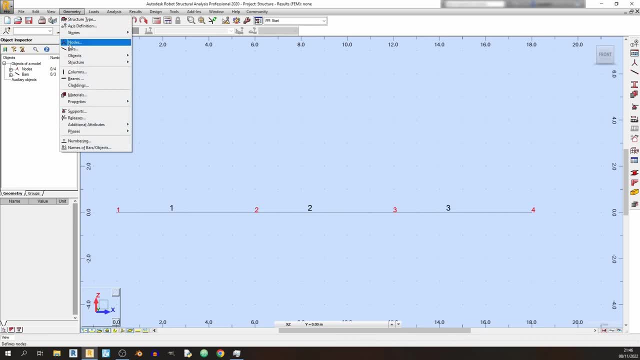 quick tip for the bar elements is that if you made a duplicate on accident, just go to the geometry, drop down over here and go to properties and sections and you can actually delete any member that you feel is no longer required. So, for example, if I want to delete this rectangular beam over here, 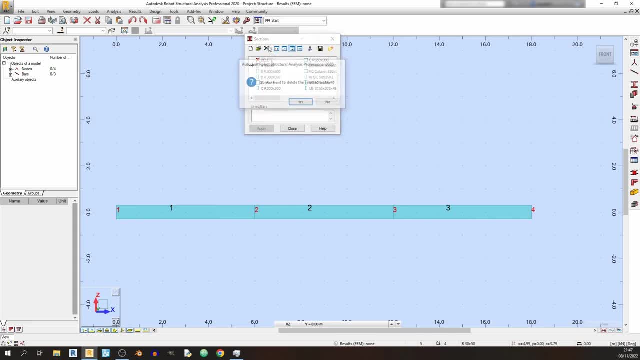 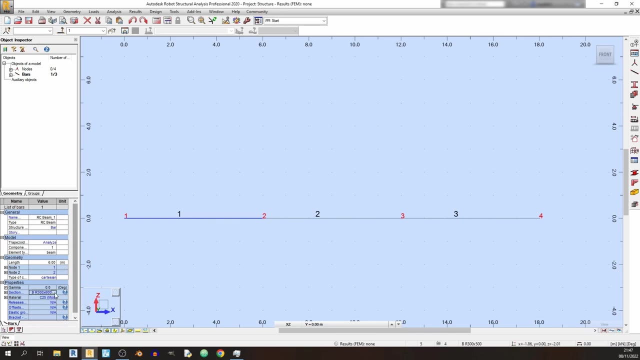 I just select it and click on delete section over here and click on yes and it's deleted, like so. And another useful tip is that if you chose the wrong section type for your bar, you can just select it and change it over here. You can choose from the drop down whatever. 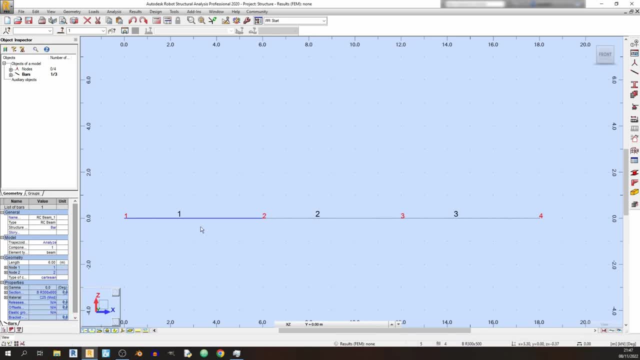 beam that you have in your analysis file. So that's another tip right there. So now let's move on to the next tip. So now let's move on to the supports for our continuous beam. So to find the supports, all you need to do is look for this particular symbol over here, Hover over it. 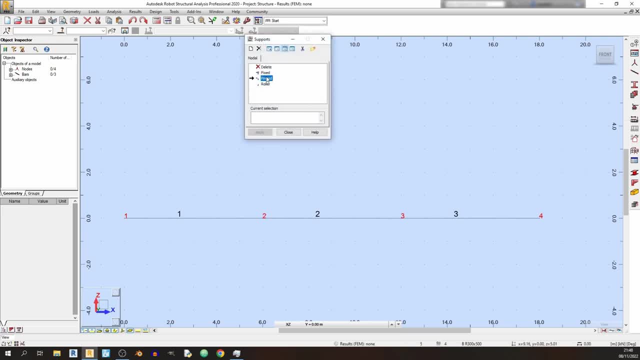 and it will say supports and choose the pinned option and I will place it at all the nodes over here and click on close. So now let's define the loads for our continuous beam over here. So click on the load types over here and we will have one dead load and three live loads. 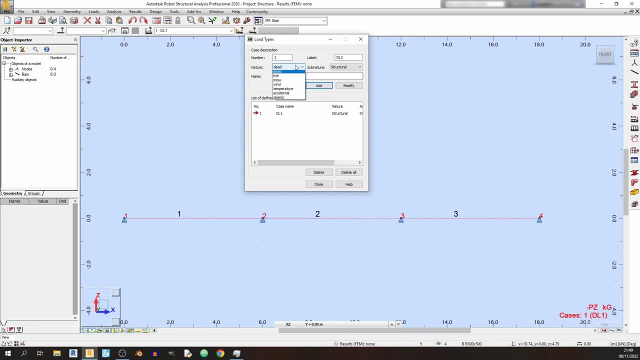 So click on add over here for your dead load and let's change it to live load now by clicking on this nature drop down and selecting live and click add three times. Okay, so we have one dead load and then three live loads. and click on close To access the load tables. you can just right click and 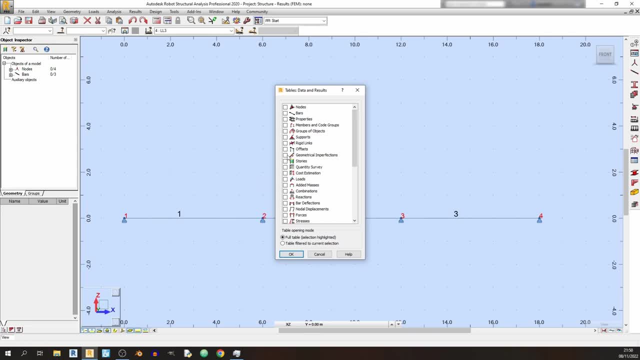 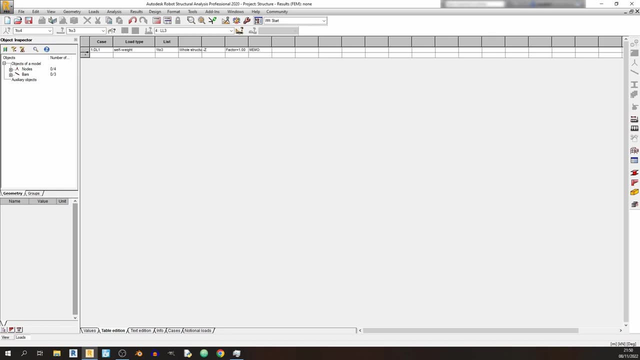 go to tables over here and choose loads over here and click on ok. So this table will emerge and, as you can see right now, the only load that has a magnitude right now is the dead load, which is currently defined as the self weight over here. So for this tutorial, 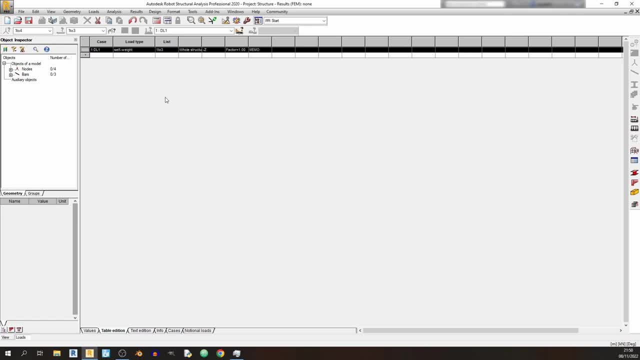 I will not be using the generated self weight and I'll be deleting it. Instead, I'll be creating a user defined dead load instead. So, to move back to the beam that we've just drawn just now, go to the view tab over here in the bottom left and you can see the 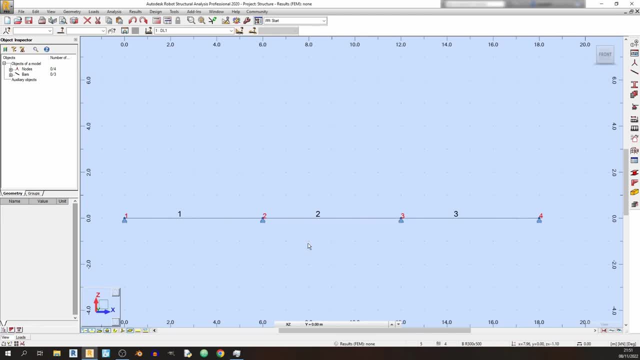 beam once again. So now let us actually apply the loads onto this continuous beam over here. So proceed to the load definition over here and click on bar. So from the diagram that I've shown you in the beginning, we will have a uniform load. 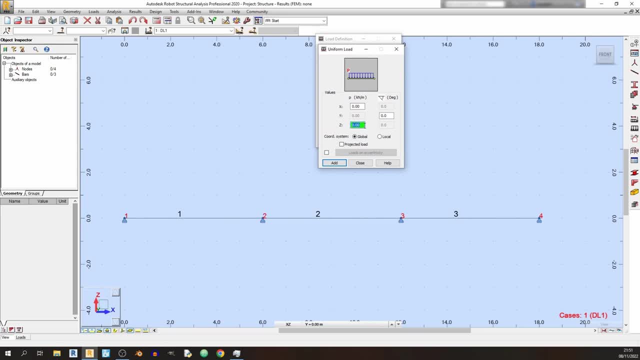 So choose uniform load over here and for the dead load we will have 25 kilonewtons per meter. So key in negative 25, click on add and select each of these bar elements here and apply And close So you won't be able to see the dead loads being applied. 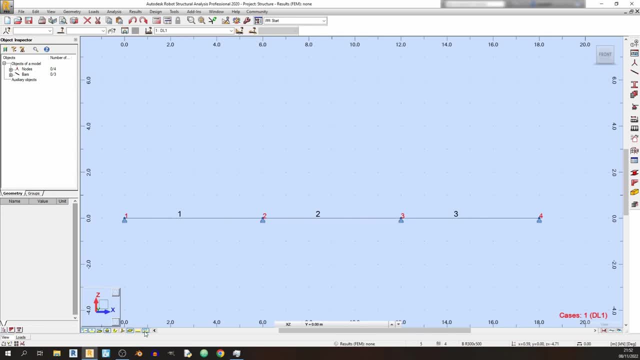 but you can click on load value descriptions here and load symbols and you can see the dead load is already applied and the magnitude is negative, 25 kilonewtons per meter. If you forgot the negative sign, the load will be acting upwards instead of downwards. So that's one. 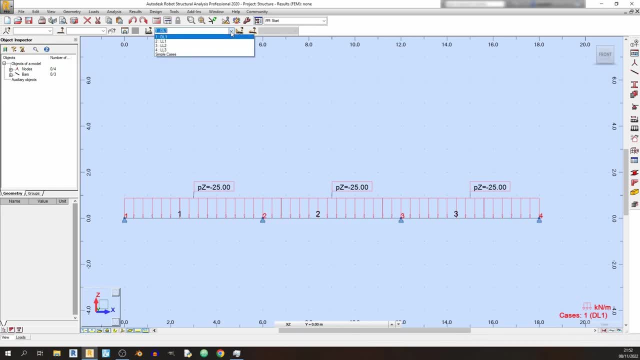 thing to note. And now we must go to the live load cases over here. So for live load 1, I will have a 10 kilonewton per meter load for bar 1 over here. So click on load definition over here, choose bar and change it from minus 25 to minus 10.. 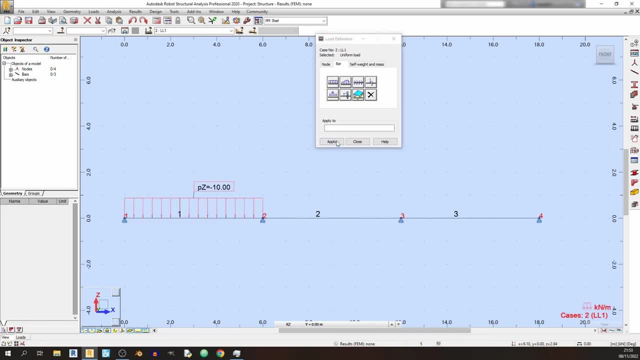 Click on add and select bar 1 and apply and close. So this is the live load 1 case over here. Moving on to live load 2, the magnitude will still be the same minus 10.. But I will apply it to bar number 2 over here and you don't actually have to. 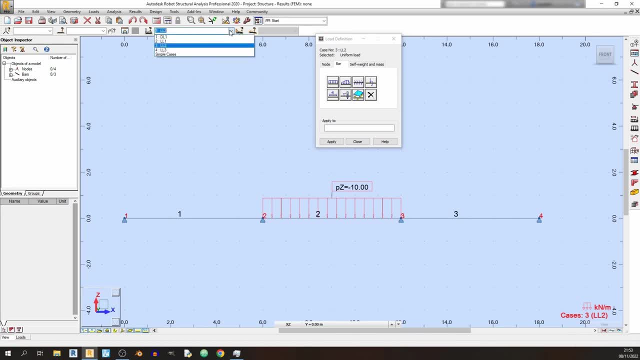 close the load definition window over here You can actually just change to different load cases and apply the loads like so. So now, if I were to change from dead load 1 through to live load 1,, 2 and 3, you can see that I've applied the loads for this continuous beam. 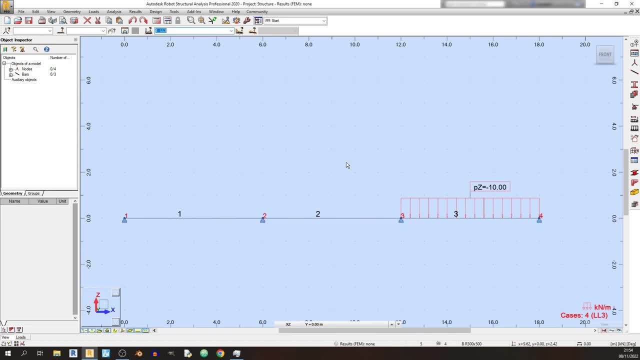 So the next phase in this tutorial would be to show you how to do the load combinations. So go to the loads drop down over here and click on automatic combinations over here. So for this tutorial I'll be using BSEN 1990-2002 National Annex. So if I click on the drop down, 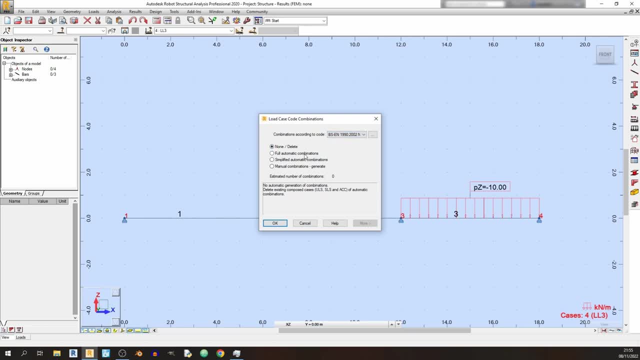 I have selected it already and I'll use the full automatic combinations over here and click on more over here, and I will uncheck on SLS accidental actions over here and fire and click on generate. So now let us proceed to the analysis of this continuous beam. So click on. 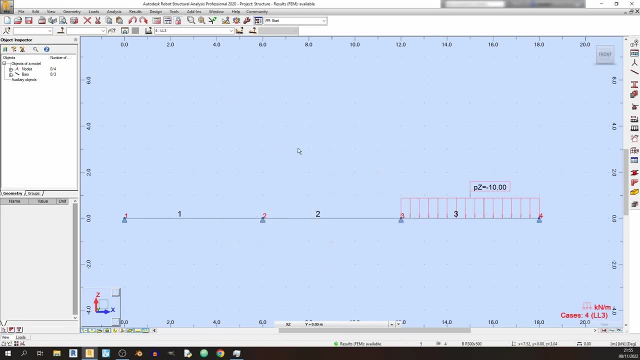 calculations over here And you shouldn't have any issues whatsoever. If you do, then you probably have to remodel your continuous beam. If not, now you can proceed to the results. So now let's quickly view the results for our analysis. So go to the results, drop down and 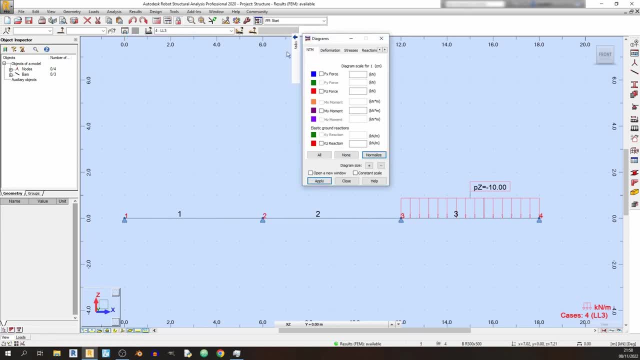 click on diagrams for bars, Go to the parameters tab over here, and I like to have the text displayed either at all locations Or global extremes. So let's say that I want it to be displayed at all locations here And in general I prefer to have it differentiated between positive and negative bending moments. 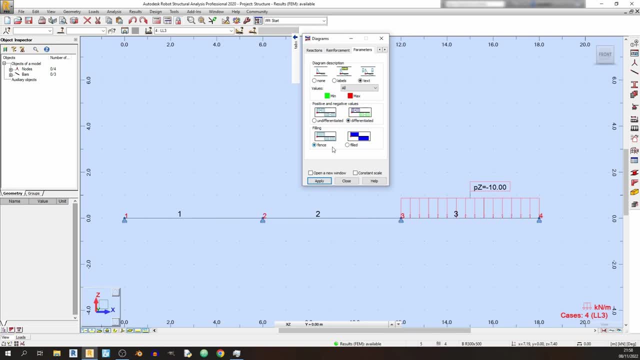 for example. So I'll choose differentiated, and you can either choose fence or filled, whichever you fancy. So I'll just use filled for now. Click on apply. Go back to NTM and I will choose MY moment over here and click on apply. 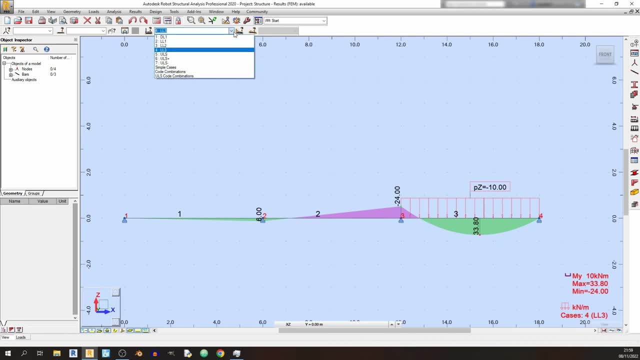 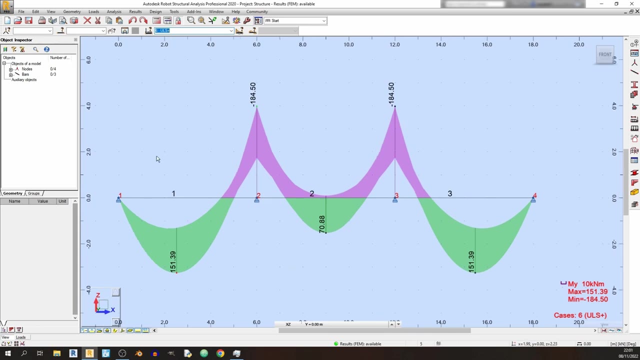 And close. So let's click on the drop down and we are interested in the ULS over here. So this is the ULS results over here. And let's try ULS plus over here. So this is the result from the ULS plus analysis. 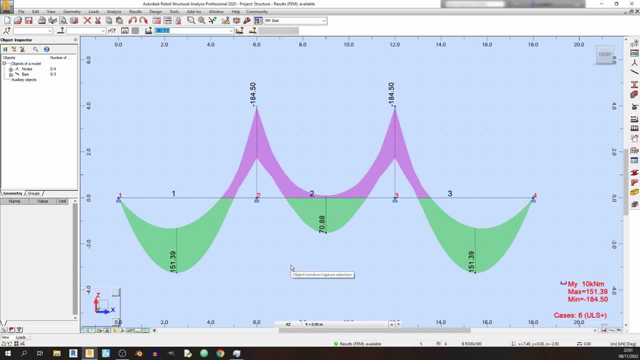 for the ULS plus load case over here. So in another video I'll be showing you how to actually check these values and whether or not they are in line with hand calculations, by showing you how to use the bending moment coefficients. So stay tuned for that. 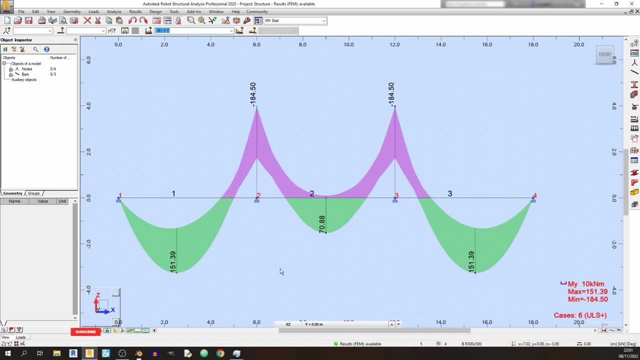 If you enjoyed this tutorial, like this tutorial and share this tutorial and subscribe for more Autodesk software tutorials and civil engineering tutorials. If you're looking for textbooks that I have used before in my undergraduate studies and in my career, feel free to contact me for those.